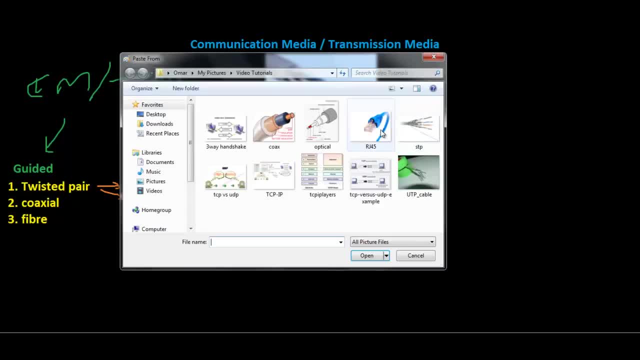 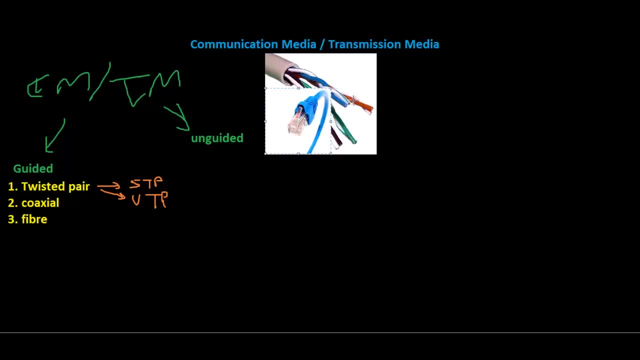 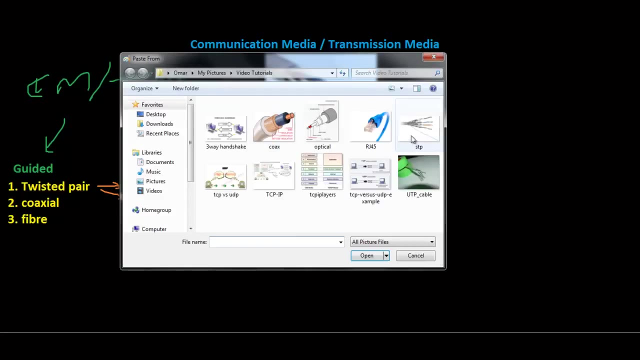 I'll show you an example of the RJ45.. We use it a lot when we are setting up our network. This is the RJ45 connector These wires would connect. Now, the shielded twisted pair is kind of similar to the unshielded twisted pair, but it has a separate insulation material between each pair. 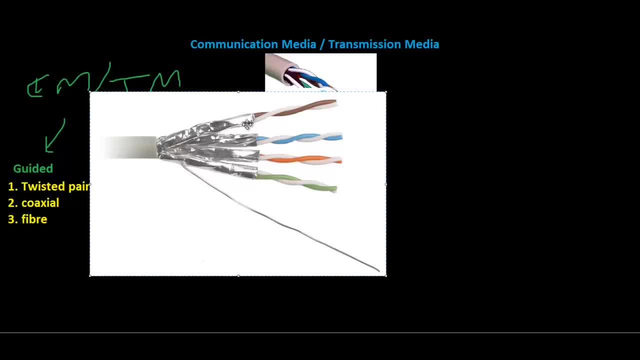 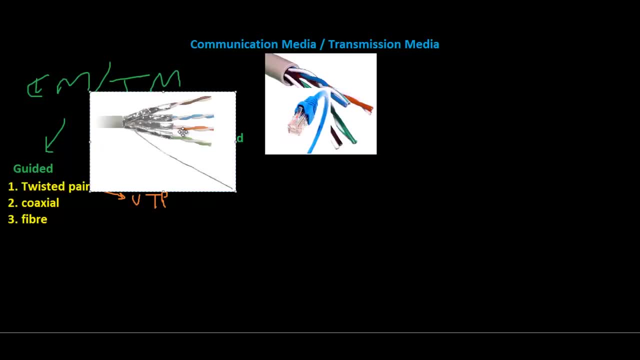 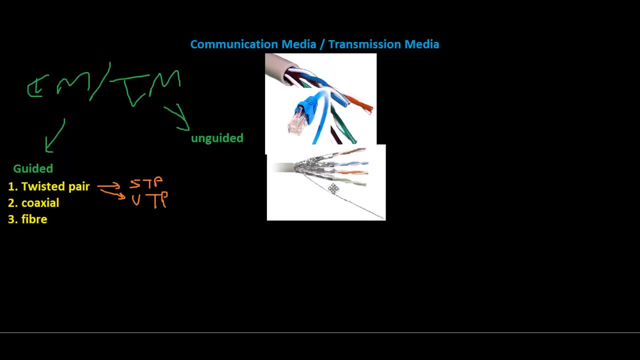 As you can see right here, each pair of wire has an aluminum foil insulator. This further prevents crosstalk or interference. Crosstalk is when the two wires interfere with each other. The shielded twisted pair is normally more expensive than the unshielded twisted pair. 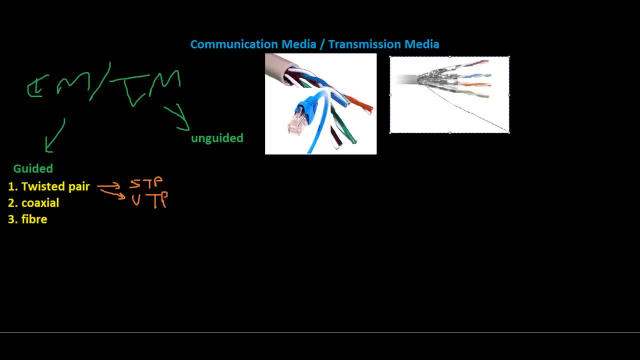 Now the shielded twisted pair or the unshielded twisted pair. rather, it's broken down into five categories Now. the first is category one. The category one: cables are used in telephone wires. It's used for voice. The category two, or cat two, they are used to transmit data up to four megabytes per second. 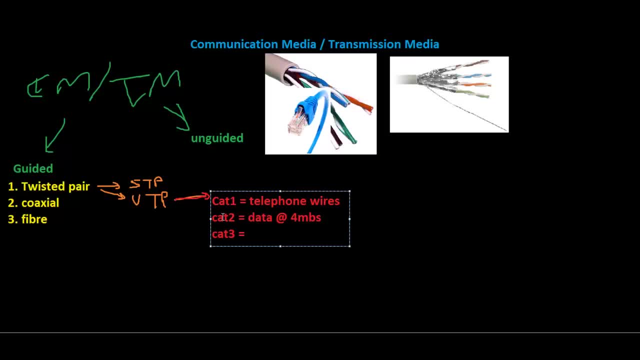 So data at four megabytes per second. Cat three is used to transmit data at 10 megabits per second, or ethernet Ethernet at 10 megabits per second. Cat four- this is token ring use to transmit data up to 20 megabits per second. 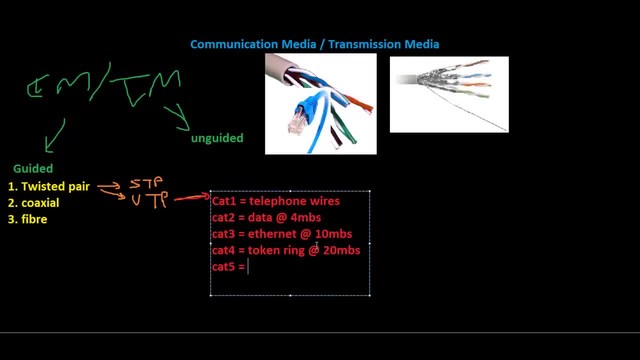 And cat five or fast ethernet- Fast ethernet, which is what we really use in our homes to get the internet. It transmits data at 100 megabits per second. As I said before, the shielded twisted pair is usually more expensive than the unshielded twisted pair. 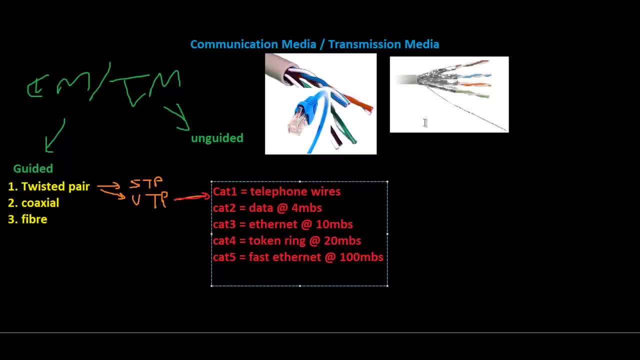 Because the shielded twisted pair is shielded, it allows the cable to run longer lengths than the unshielded twisted pair. Next added media is the coax. Let me show you an example of the coax. I think we're all familiar with the coaxial cable. 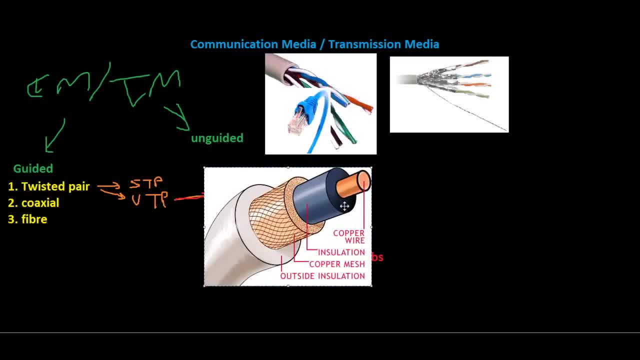 The coax cable has a central conductor, which is here Normally copper. It's surrounded by an insulating material- This is normally called a dielectric material, And then it's normally dielectric, is surrounded by a copper mesh, And then everything is encased in an outside insulation material. 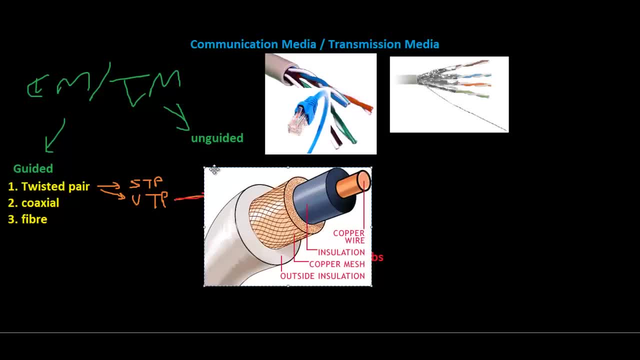 Coax cable. it allows runs of distance of up to 500 meters and can support up to 100 nodes On a network. It's very resistant to interference. Coax is more expensive than the twisted pair cables, Fiber or optical fiber. 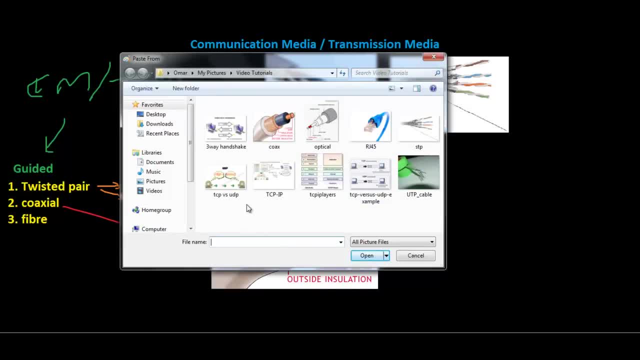 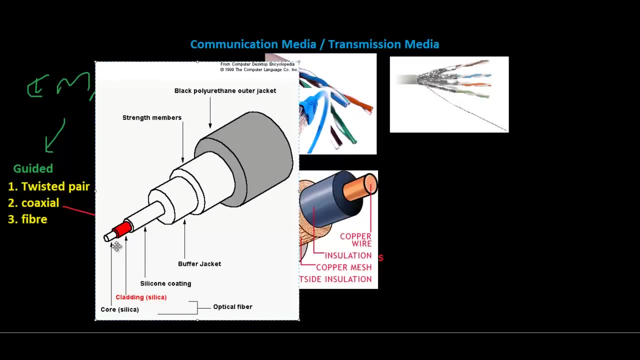 This uses light pulses rather than electrical signals to transmit data. Normally made of glass or plastic, It has a small silicone core, So it has a small silicone core. The core is normally made of silicone And encased in some light absorbent material. 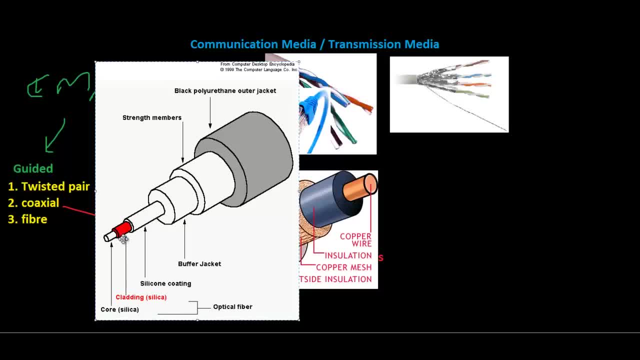 Plastic called cladding. So this is the cladding. It has further insulating materials. So, as you would probably imagine, this type of media is hard to tap into penetrate Because once you break the core then the signal is lost. 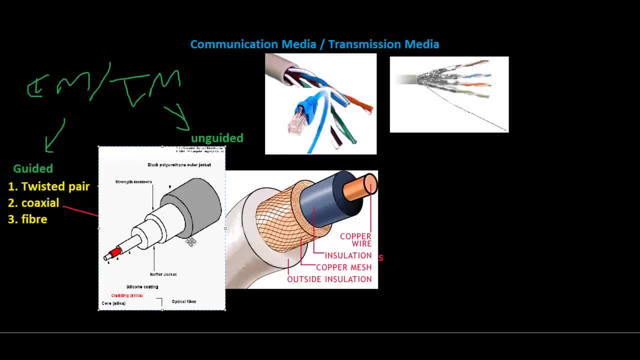 It's much more secure than the two other categories of transmission media. There are five forms of optical fiber. First one is the multi-mode- Multi-mode mode, This: With this form of optical fiber, The light comes in at a variety of angles. 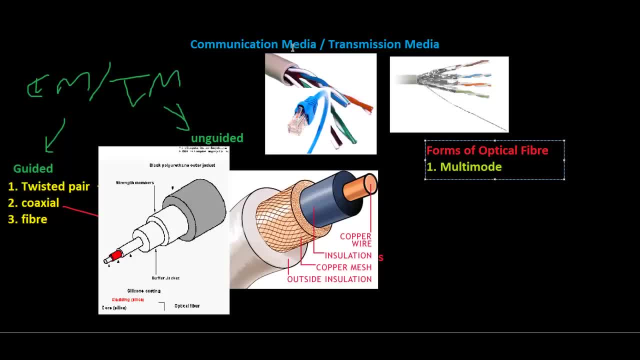 And the bandwidth is less than 200 megahertz. Let's use B to represent bandwidth. The bandwidth is less than 200 megahertz. The second form is known as a multi-mode graded index. With this mode, The fiber bends signals as they approach the cladding. 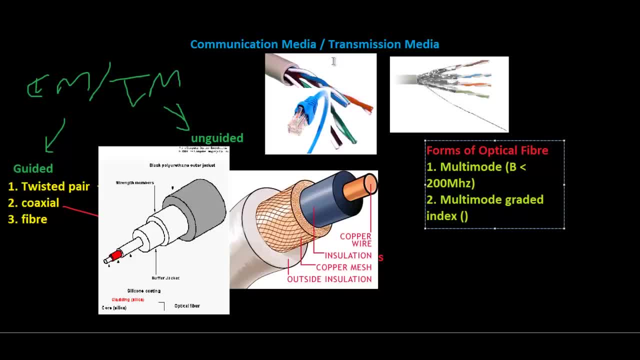 Instead of reflecting them. This supports a bandwidth Between the range 100 megahertz to 3 gigahertz per kilometer. So B at 100 megahertz, 3 gigahertz per kilometer. Our third mode is called the single mode. 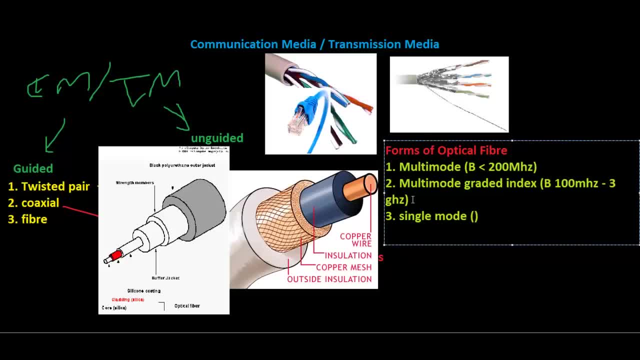 Single mode. It's normally supposed to be the highest bandwidth Because the diameter- As in this central core right here- Is reduced Only allowing one light signal to pass. It supports bandwidth up to 50 gigahertz per kilometer. Fourth mode is the breakout cable. 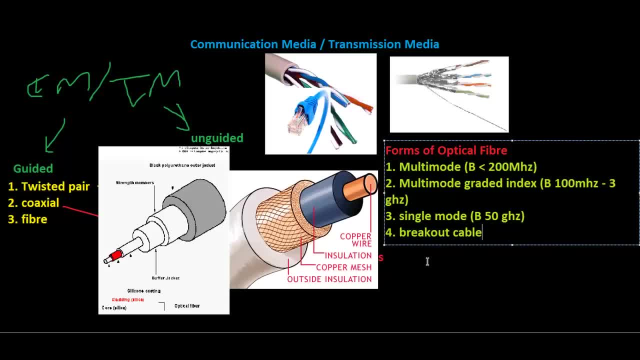 Breakout cable. This has several fiber. Each has its own cladding And a jacket surrounded by a larger jacket. What this means? Let's say this is the fiber. I don't have the example. Okay, Let's say this is our fiber cable.